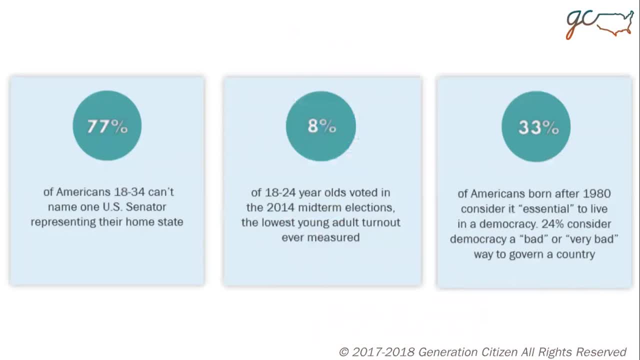 What about your US Senator? Can you name them? Could your students name theirs? 77% of Americans 18-34 can name one US Senator representing their home state. Let's talk about voting. Do you vote? Only 8% of 18-24 year olds voted in the 2014 midterm elections- the lowest young adult turnout ever measured. 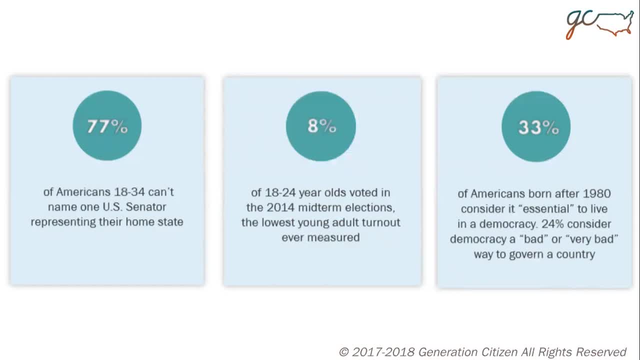 You start to understand why this might be the case when you learn to vote. I learned that only 33% of Americans born after 1980 consider it essential to live in a democracy and 24% consider democracy a bad or very bad way to govern a country. 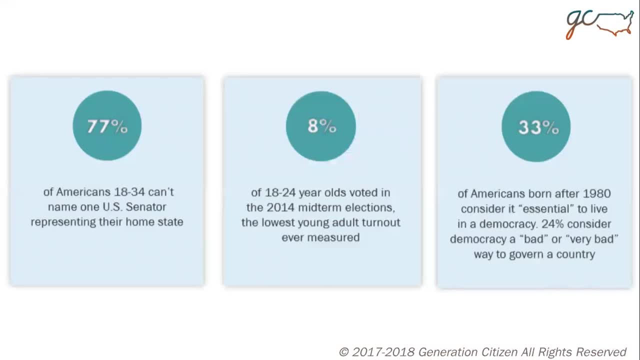 What we are seeing in turn is that young people are turning away from the political process. Though 64% of millennials say it is a priority for them to make the world a better place, only 20% trust the federal government to do what is right. 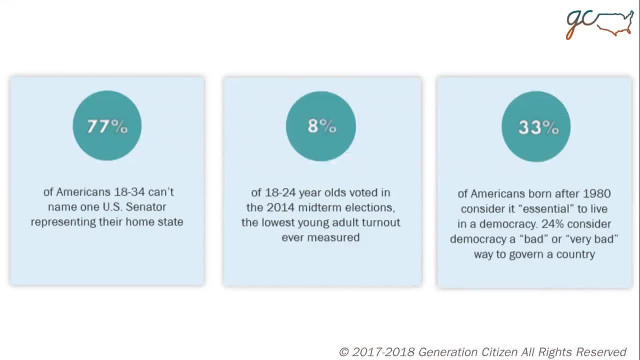 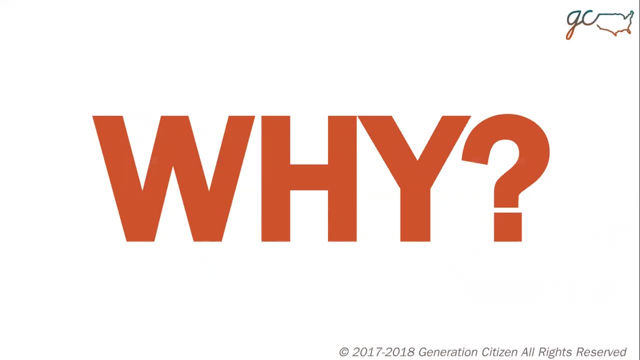 Those are some hard numbers to swallow. There are many reasons why for the lack of informed youth, political engagement and belief in democracy. One of the biggest reasons is the failure of our nation's schools to achieve one of their founding purposes: educating young people to be engaged, informed and responsible citizens. 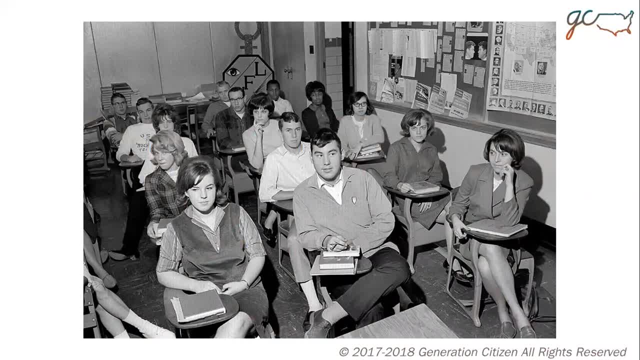 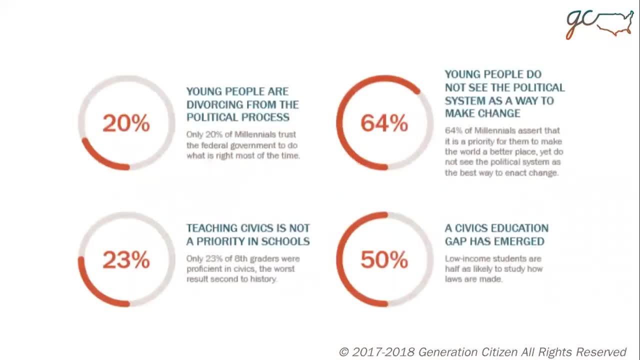 It didn't used to be like this. In the 1960s, three separate courses on American government were common in US high schools. Today, if civic education does still exist at a school, it most often deals solely with rote historical and governmental knowledge. 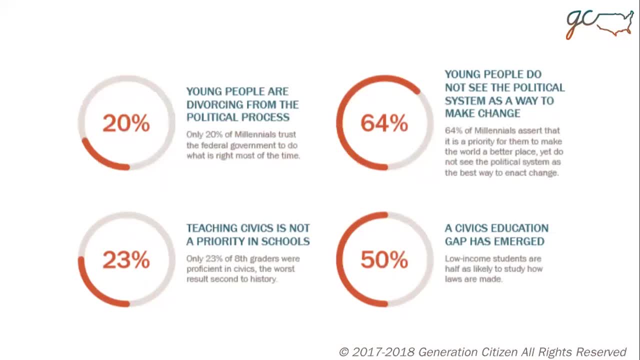 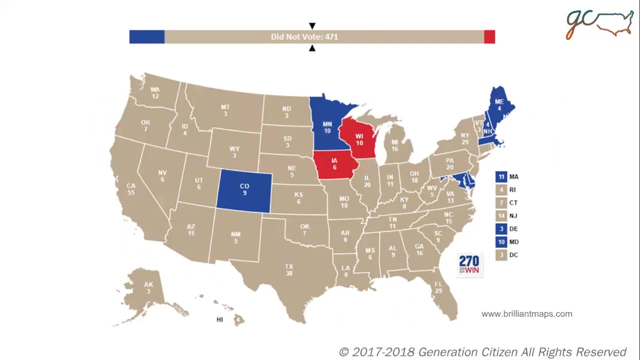 What's more, the civic engagement gap has worsened, with the low-income communities less likely to receive effective civic education experience. As a result, young people are rapidly divorcing from the political process altogether. They're not the only ones not participating.